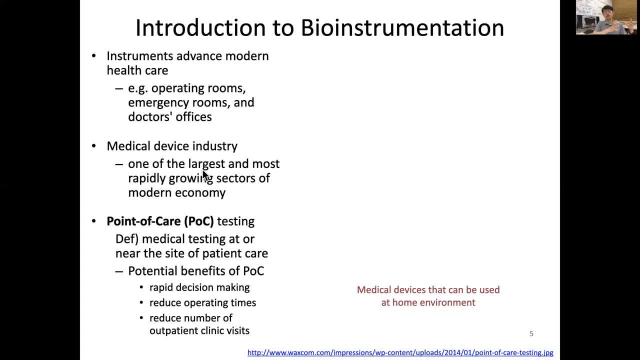 So for that there is a tendency that these bulky, big, very costly instruments inside a clinic or doctor's office and that tend to be smaller and portable and it's available at a lower cost. So that's why we call it a point-of-care or POC testing, which means the medical testing at or near the site of patient care, like patient's home. 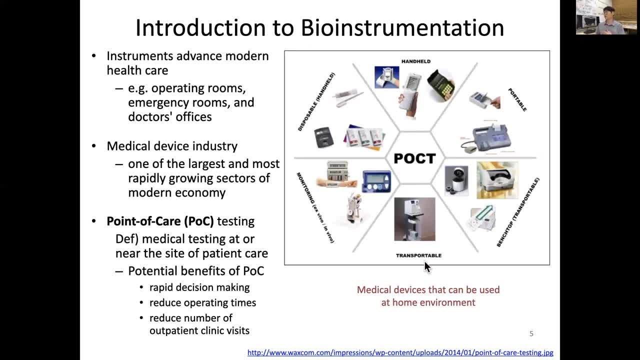 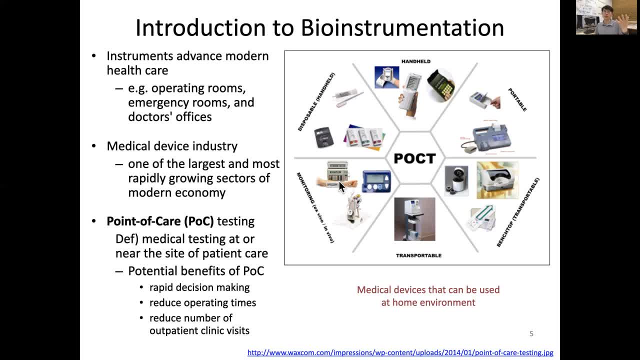 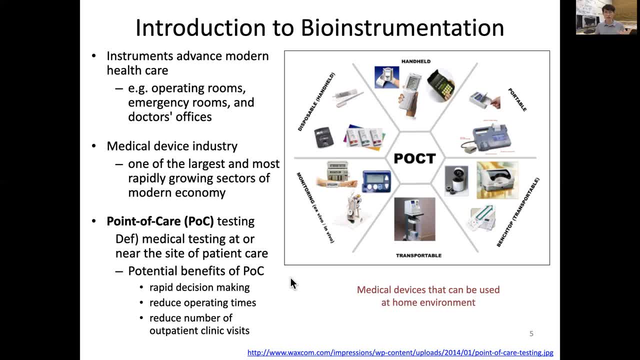 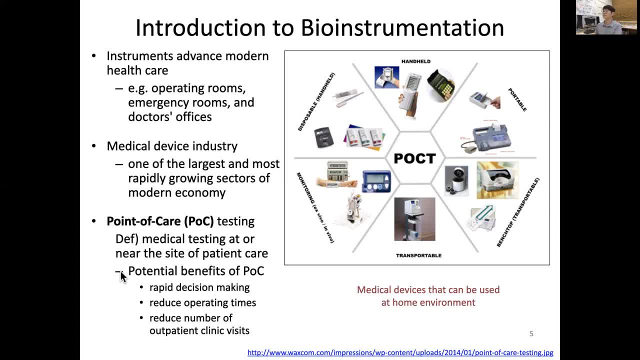 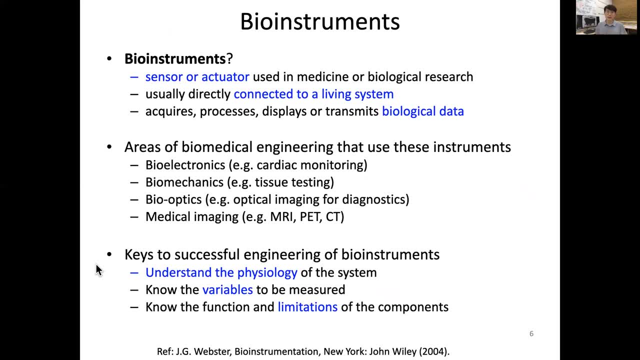 So let me show an example of a point-of-care testing device, which is now more transportable and monitoring device for patients and displays and transmits the biological data. So areas of biomedical engineering that uses these instruments are many, So, for example, bioelectronics. 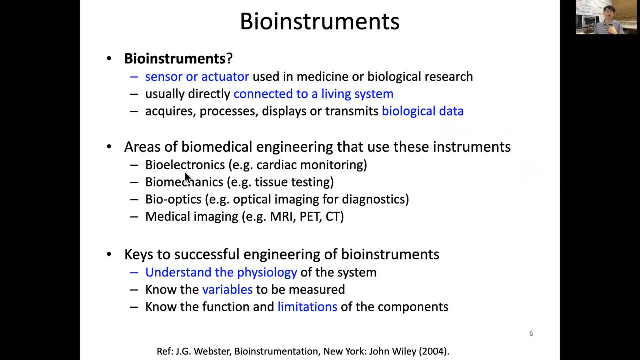 and good example is cardiac monitoring or ECG, EKG monitoring device and biomechanics which measures, for example, tissue testing or like long respiratory function test. Another example is a bio optics, which is a optical imaging for disease diagnostics. A good example is an endoscopy: optical endoscope And medical 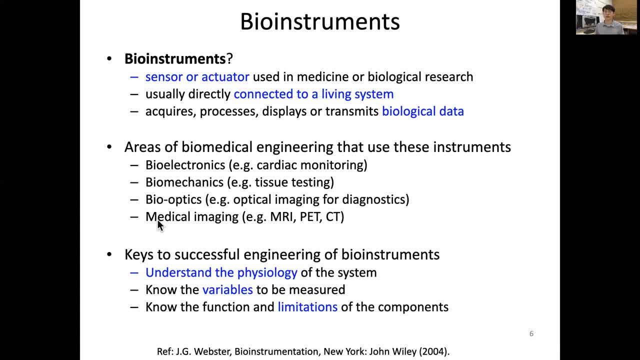 imaging is also another areas of using this instrument, such as MRI, magnetic resonance imaging, cat positron emission tomography and CT, which is x-ray computed tomography. These are like kind of instruments, So for the keys to successful engineering of bio-instruments, where we first need to understand the 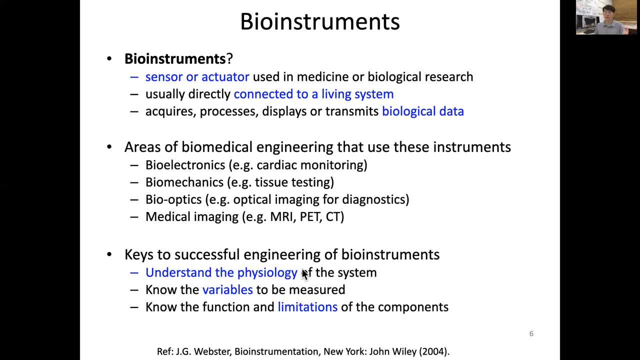 physiology of the system, The biological system or the patient, and the pathophysiology, the physiology of the diseased organs or function of the system. And for instruments we have to know that it is in the system that the disease or the pathophysiology can be. 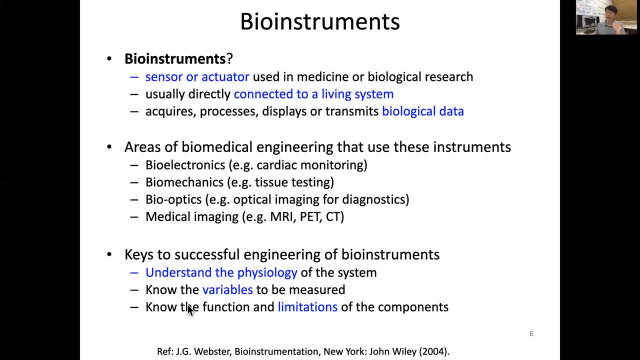 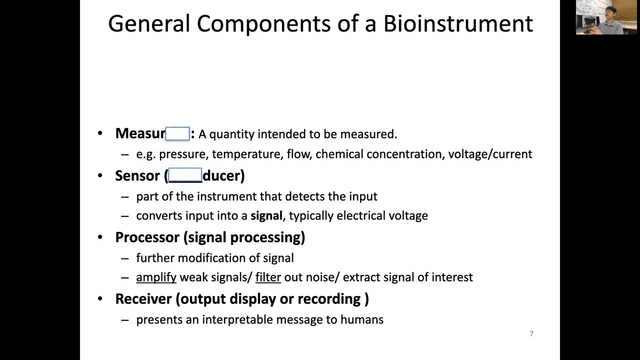 the variables to be measured, and also knowing the function of the components of instruments and also, very importantly, the limitation of the instruments, for example, the range of values which is reliably measurable by the instrument. you have to know for this. so now let's discuss about general components of bio instruments. 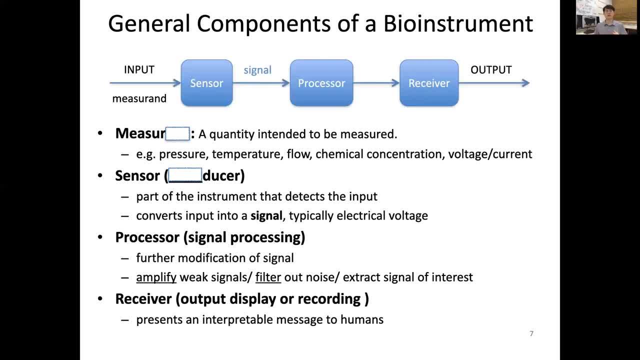 so here it's a diagram showing. so we have an input. so which is we call measurement. so this is a measurement, is a quantity that is intended to be measured, so that's a measurement. uh, for example, like we want to measure blood pressure, patient temperature, uh, blood flow. 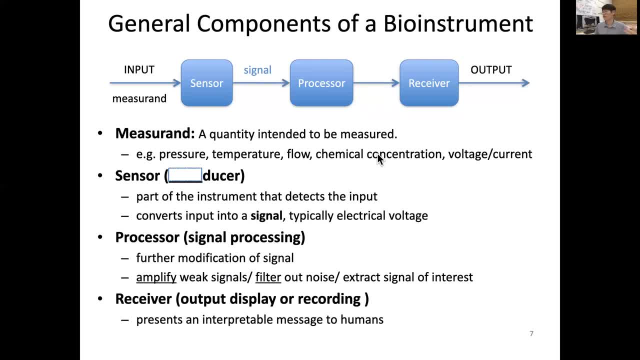 and chemical concentration or voltage current, and those are the measurements and that can be measured by sensor. so sensor is a part of instrument that detects the input and usually converts into a signal. signals are now mostly electrical voltage here, so input can be a various of physical entity or electrical entities. 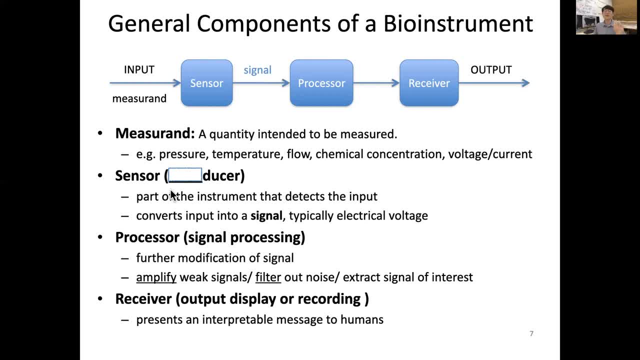 that that converts into electrical voltage. so sensor is on the other way, it's called as transducer. so you remember, in cell signaling pathway there is a signal transduction pathway. we call because transduce means converting one type of signal to another type of information. so sensor is a transducer. now you convert it into. 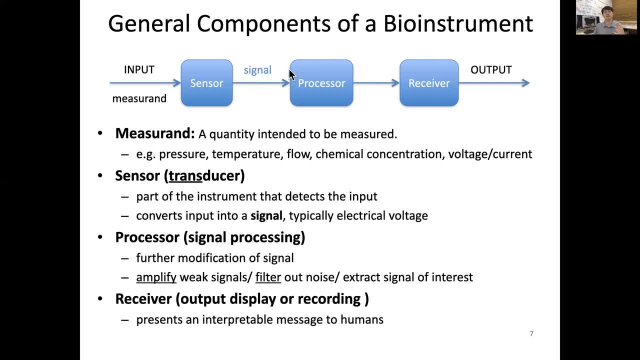 a raw signal, then there needs a processing for a process for the raw signal. so further modification of the signal, because many times the signals are so weak that you need to amplify the signal also. at the same time. signals usually comes with a noise, so you have to. 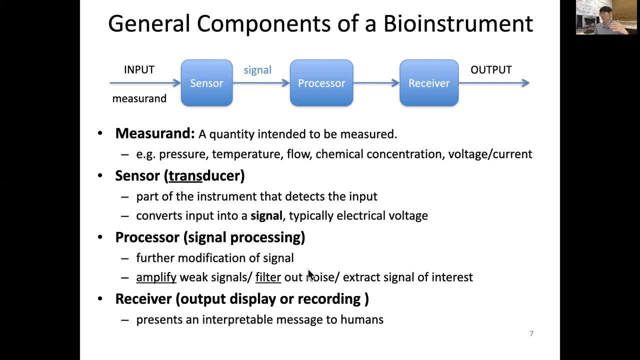 sometimes condition, filtering the out the noise and signals there are, like your interest, signal of interest you can extract from the signal and then you can control these collectively as we call signal processing. and after this signal processing we need to get into the receiver, which is example like output display or 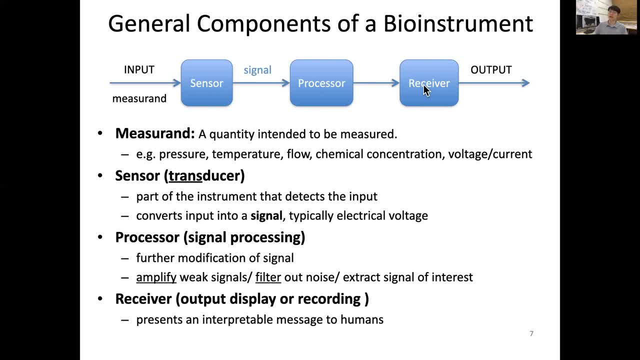 recording. so the it presents an interpretable message to humans or clinicians or to the patient. so, in a nutshell, input is being sensed by the sensor or transducer to convert into electrical signal and then you can process the signal and then you into the receiver to display or recall the results. 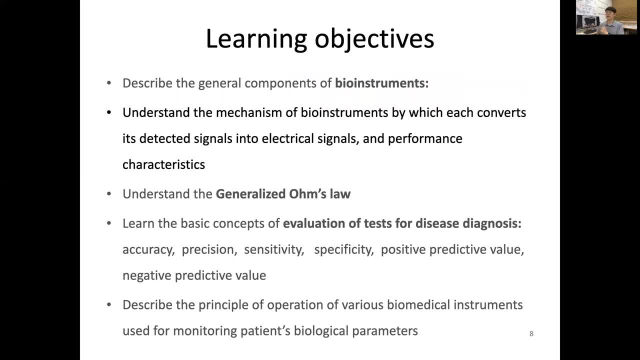 as an output. so next time we will discuss about the mechanism of bio instruments and it's detected signals into electrical signal.